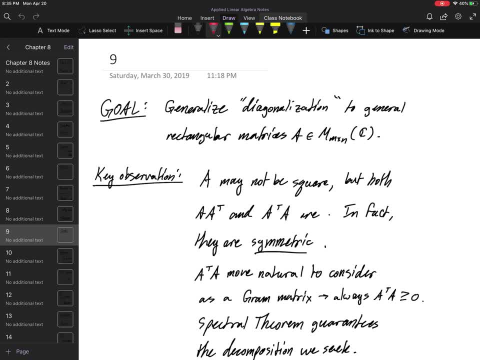 rectangular matrices, And that turns out to be a bit of a problem for us, because we only know how to come up with diagonalizations for matrices that aren't diagonalizable. So let's see if we can't find a way to just kind of skirt around that and make up for 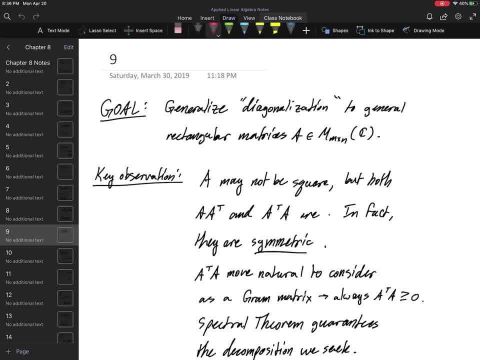 that shortcoming And a key observation we'll make is that A, even though it might not be square, both A A transpose and A transpose A are. So, more to the point, these guys are symmetric, so both of them are diagonalizable, But it's actually, you've seen in your homework. 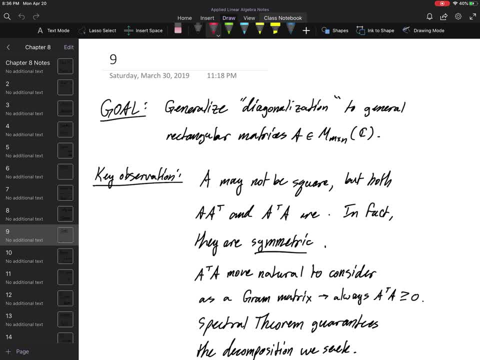 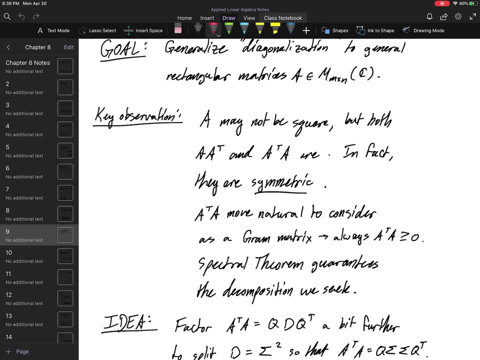 that it's more natural to get a diagonalized A transpose than a square, because it's more linear than a square. So we're going to consider A transpose A in this case, because this guy is always positive, semi-definite at the very least. So it is a positive matrix, A transpose A. So the matrix. 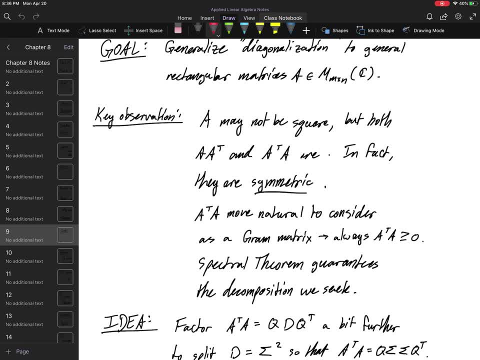 A times A transpose is going to be more of what we call a projector matrix, And again, you've seen this in your homework- that A times A transpose really corresponds to a sort of orthogonal projection. But we won't worry about it right here. We're going to take a 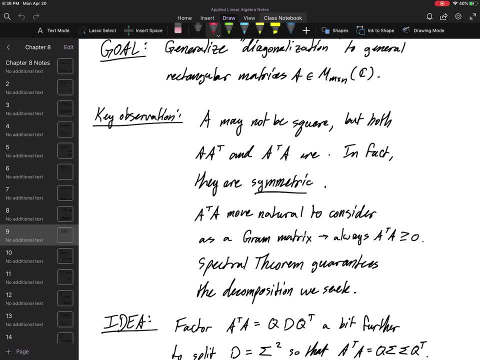 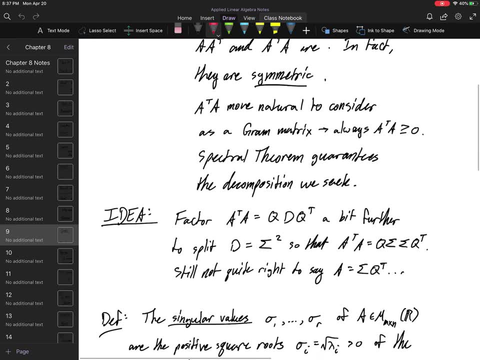 look at the Gram matrix, And then we'll take a look at the A transpose A matrix, And then we'll look at A transpose A, because this guy is symmetric and he's positive. The spectral theorem then guarantees a particular decomposition of this matrix. So it may not be a decomposition of A that we'd come up. 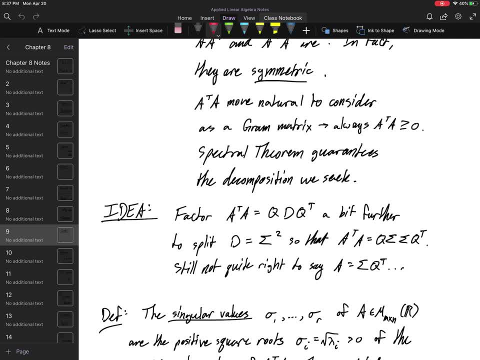 with in this case. but we can kind of force ourselves into a decomposition for a matrix related to A, And what we're going to do is factor out exactly A, transpose A into its spectral decomposition And this will be effectively the diagonalization that we know and love. 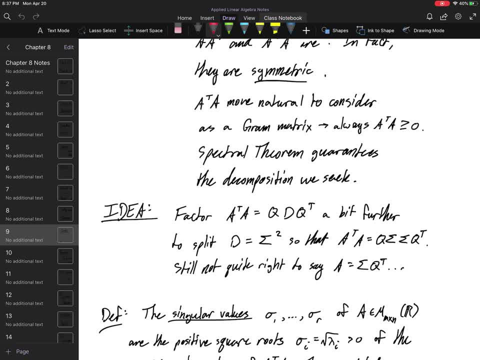 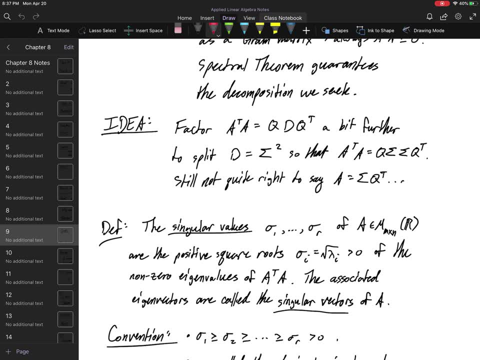 So in this case we are going to go a little bit further here. So what we would like to say is that, okay, we have the decomposition that we want for A kind of hidden in here in this. Q times, D times Q transpose matrix. 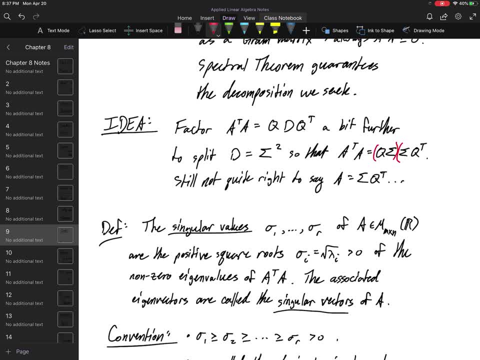 And the idea would be to split this guy up into two very similar pieces, And in fact these guys are transposes of one another. So really we would like A to just be the right-hand portion of this decomposition, But it's still not quite right to say that right. 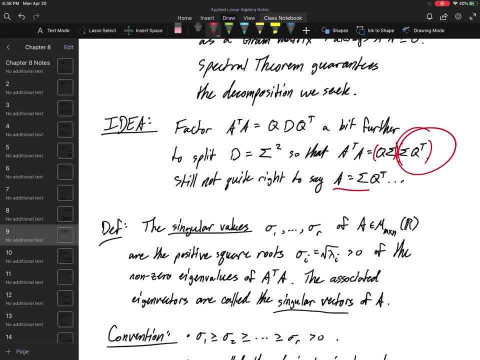 Because this is definitely not the case. right A is not equal to this. sigma times Q transpose. These guys may not even be the same dimension. So we need to find a way to solidify that idea, but make it a little more rigorous. 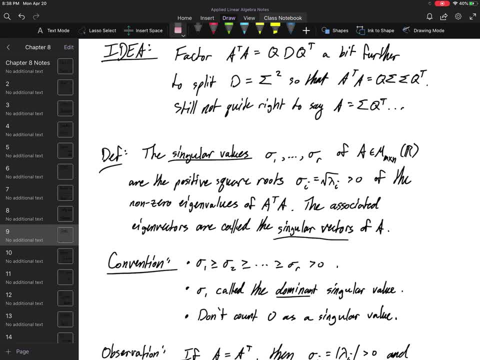 Try to find the correct way of splitting up A transpose A into pieces that look like A and A transpose respectively. So we're going to go ahead and define the singular values of the matrix. A And A is just an arbitrary rectangular matrix For right now. we're going to consider real matrices. 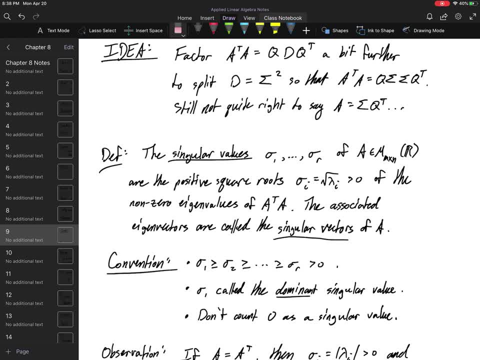 There is an argument to extend this to complex numbers, But we're not going to. We're going to worry about it for right now. So the singular values, sigma 1 through sigma r- So notice r- may or may not actually be equal to the rank. 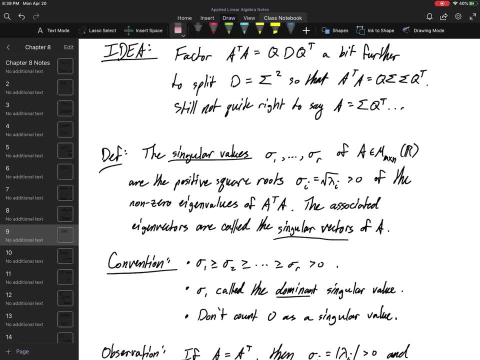 Or sorry, it may not be equal to the minimum between m and n, But these singular values are the positive square roots of the non-zero eigenvalues of A. transpose A, So the non-zero elements of this D matrix upstairs are going to be kind of our analog, for 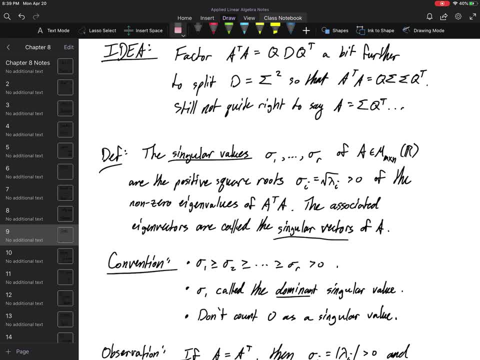 for the matrix A, Or at least their square roots, will be the analogs of eigenvalues for A. The associated eigenvectors that we get here are called the singular vectors. So, again, these singular vectors are not going to correspond to any null spaces. 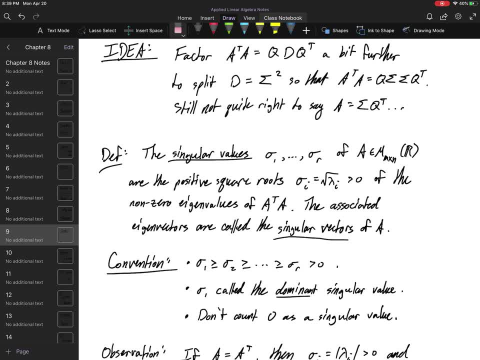 We need to make sure that all these singular values are positive numbers. Therefore, none of these sigmas are going to correspond to the null space of A. We need to make sure that all these singular vectors are going to correspond to the null space of A. 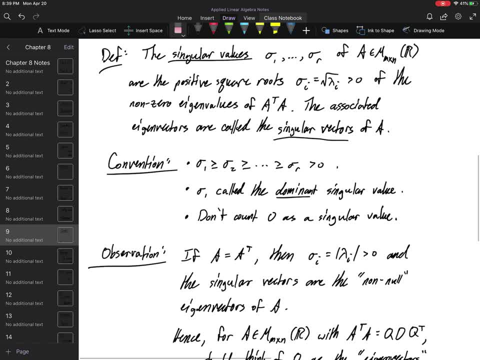 So the convention here is to line these guys up, Order the singular values from greatest to least right. So, first of all, how do we know they're all positive? Well, again, it's because A transpose A is going to give us. there he is. 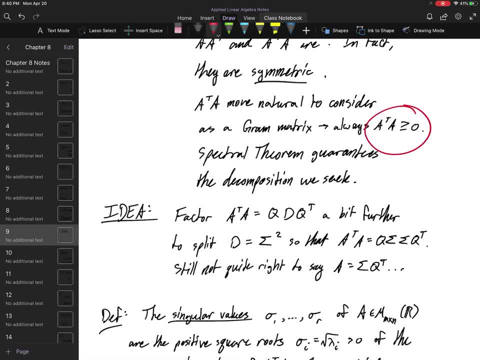 Oh shoot, did it again. A transpose A is a gram matrix, So that means that its eigenvalues are always non-negative. So we can just compute square roots. So this A transpose A has non-negative eigenvalues. Therefore, I can go ahead and take the square root of each and every one of them without penalty. 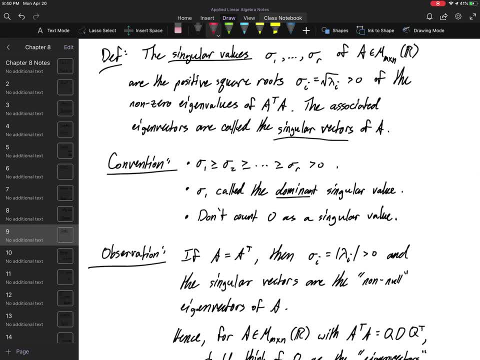 and still come up with real numbers at the end of the day. So we're going to order these guys from greatest to least, And that'll be sigma 1, bigger than sigma 2, all the way down to sigma r, And all of these guys are going to be positive numbers by definition. 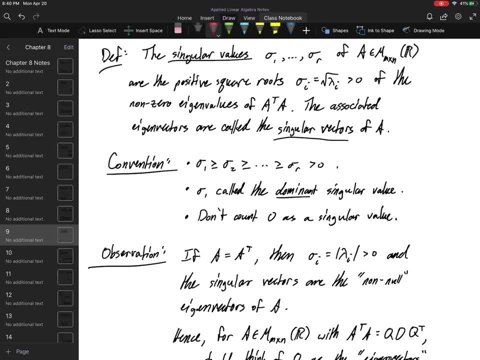 Sigma 1, we're going to go ahead and call the dominant singular value right. This guy is going to be the largest contributor to something, some property. So this is going to be the largest part of A, like the biggest part of A. 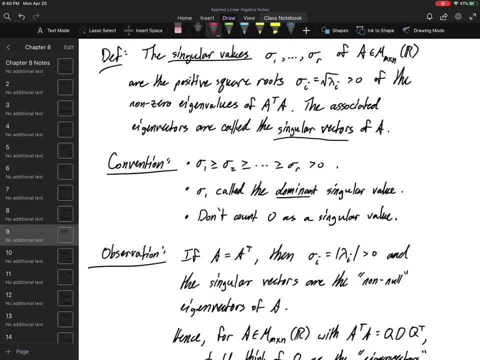 the most impactful part of A, the most dominant part of A. So we just want to make sure in this convention, that we don't count zero to be a singular value. MATLAB does this kind of, and I'll show you in a moment when we talk about the example at the end of the section or at the end of the video. 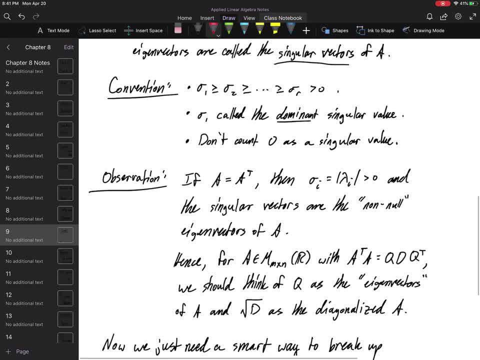 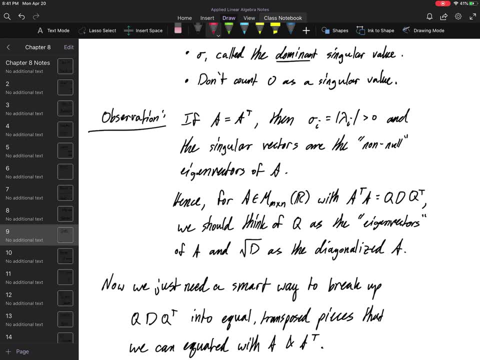 But we're going to make sure that the singular values are positive numbers And if it happens to be symmetric, then sigma is going to be equal to some absolute value of an, the absolute value of some eigenvalue. right, And you can, you know, screw it. 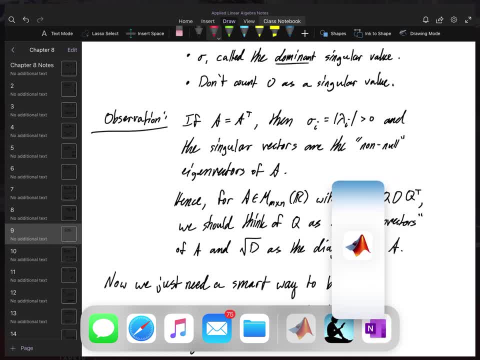 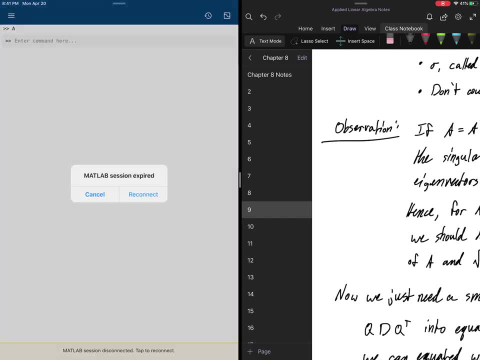 I'm going to go ahead and pull this up. No, wait, not that one. No, we're going to pull up MATLAB And MATLAB is going to go on the left side of the screen. There we go. So let me go ahead and clear that and see if it wants me to wake anything back up. 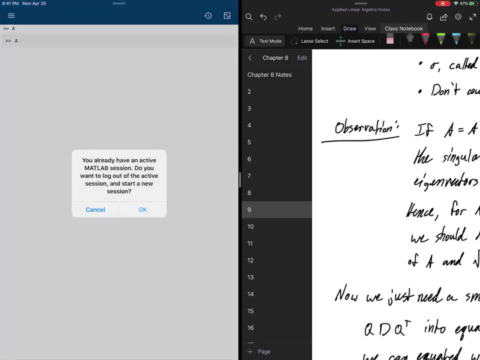 Yep reconnect. Please pay no, no mind to the man behind the curtain here. I have an active session. today I have an active session. Yes, yes, yes, Go ahead and start it. It's okay, La-di-da-da-da. 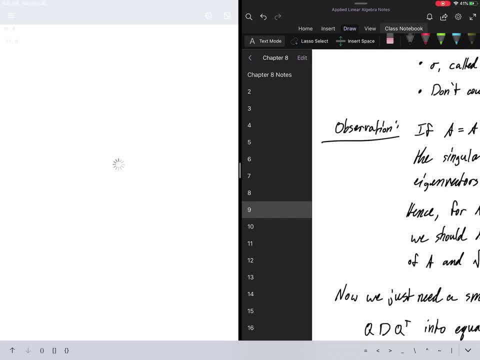 I swear. every time I begin the videos I have logged in and logged back into MATLAB, But these for some reason log me out within like five minutes. It just kills me. But anyway, the example that we're going to have at the end of the section here is this matrix given by A: 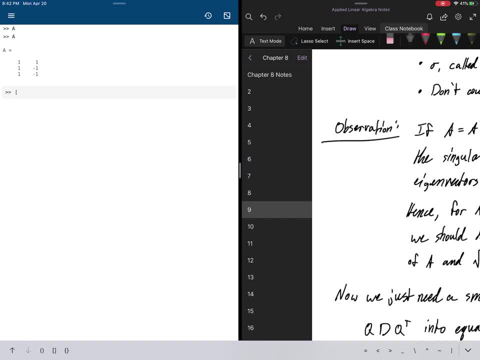 So feel free to follow along here. The command that you're going to need to know for MATLAB is just as simple as it sounds. We're going to make SVD because we're trying to create the singular value decomposition. So let me show you. 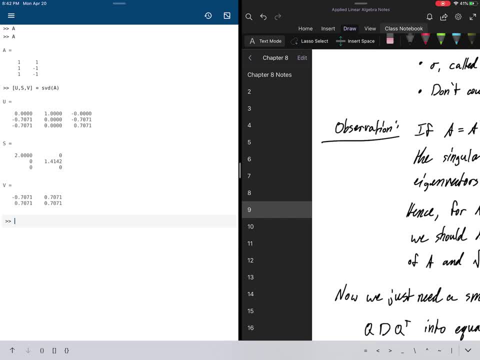 It's going to spit out three matrices for you and we'll see how they go back together momentarily, But SVD is effectively what's going to give you your eigenvalues for this rectangular matrix, And S is going to be the matrix that contains those guys. 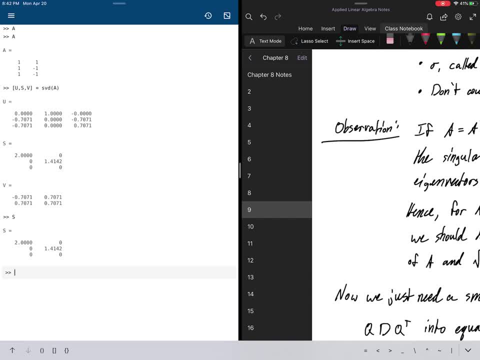 So notice no zeros on the diagonals. Right The values are positive. However, this U matrix repeats the first and third column. So that's what I mean by kind of They kind of do the right thing. We're just making sure that we zero out any superfluous vectors in this U matrix. 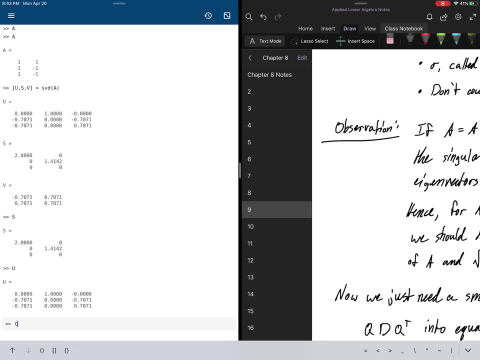 We'll talk about that momentarily. Coming back to the point at hand, let me go ahead and create this matrix: minus 4 by 1 by 1 by minus 4.. And this guy, I can go ahead and compute the eigenvalues for this. 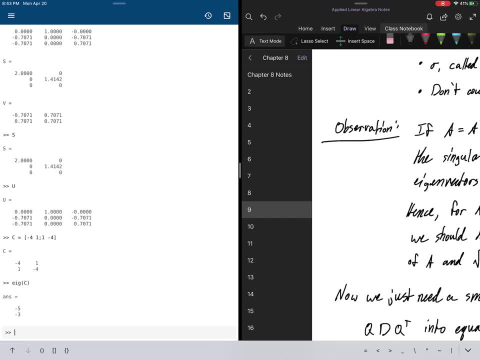 Sure, You can go ahead and compute them yourself. You know how to do this, But you can verify they're both negative. However, if I were to create little u little s little v as the SVD of this matrix C, 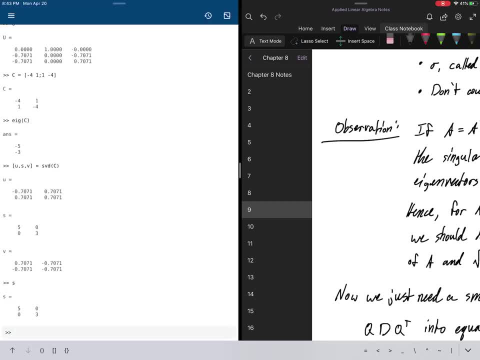 notice what happens to the S matrix. The S is still comprised of positive numbers. This is because A transpose A or C transpose C, in this case, is a Grom matrix And that is a positive, at least semi-definite, matrix. 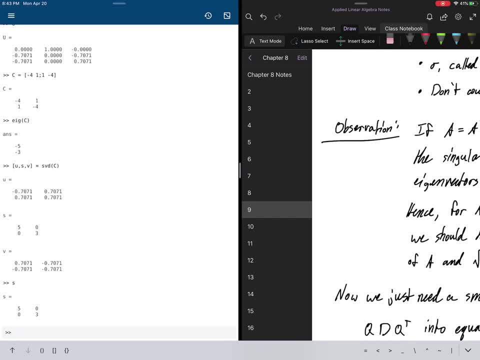 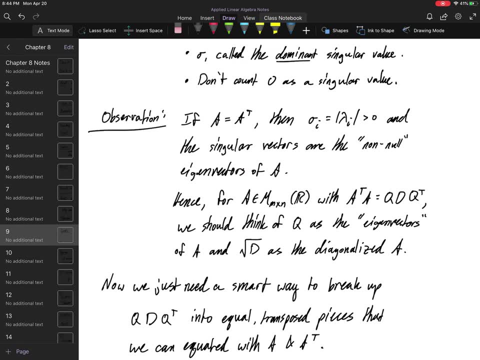 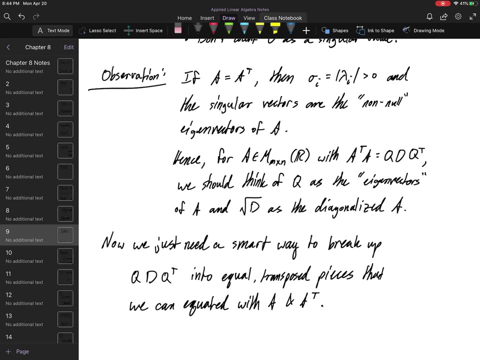 So that means that we don't quite get a diagonalization as we did before. This singular value decomposition is going to give us something that orders the dominance of the eigenvalues Right. So what we should think of here is: in the symmetric case. 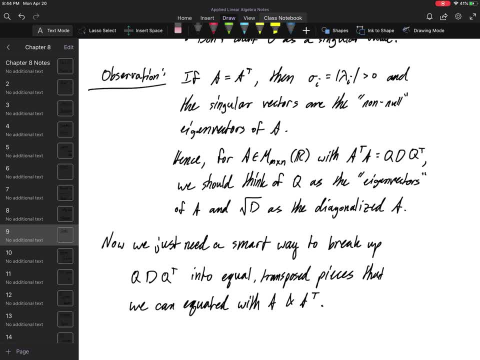 if A is equal to A transpose, then the singular values are the absolute values of the eigenvalues of A and the singular vectors are the non-null vectors. So in other words, we need to make sure that all the eigenvalues we take here 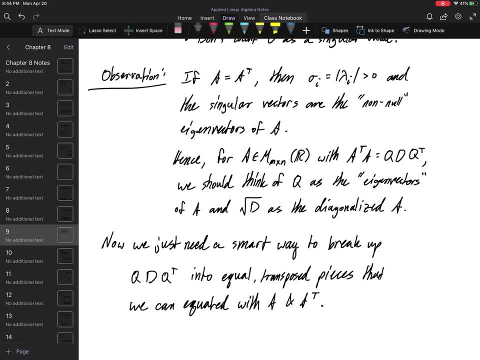 for our singular values are non-zero. So that means that we can't be using any vectors that belong to the kernel of A Right. So we're just omitting all the non-null space vectors. So for any rectangular matrix with A, transpose A equal to Q, D, Q transpose. 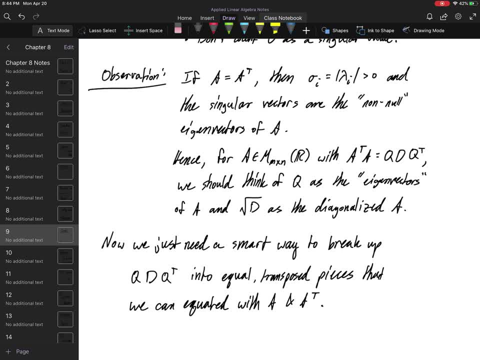 we should think of Q as containing the eigenvectors of A, And effectively the square root of this matrix. D is going to be the diagonalized version of A, So we just need some smart way to break up Q, D, Q transpose into equal symmetric pieces, or at least transposed pieces. 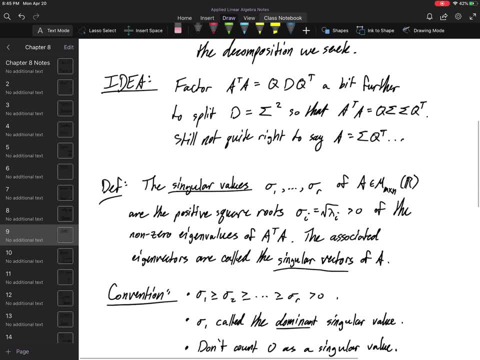 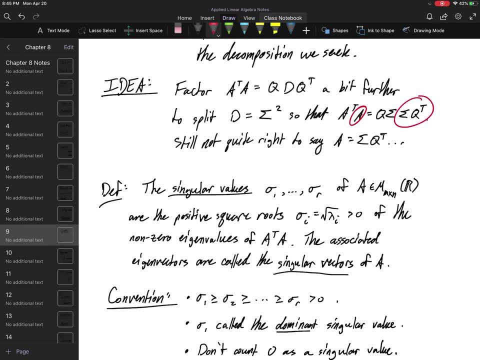 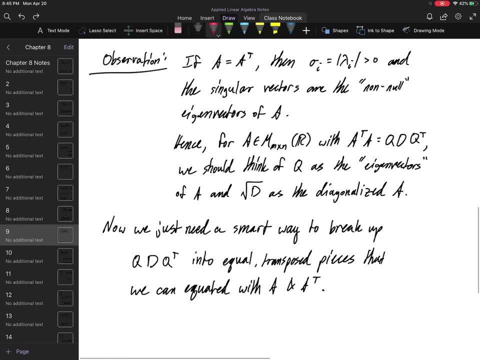 such that we can go ahead and make this connection upstairs, that this A oh shoot, that this matrix A is actually kind of linked up with this sigma times Q transpose. So let's see if there's a smart way to do this. I bet you, since I'm talking about it. 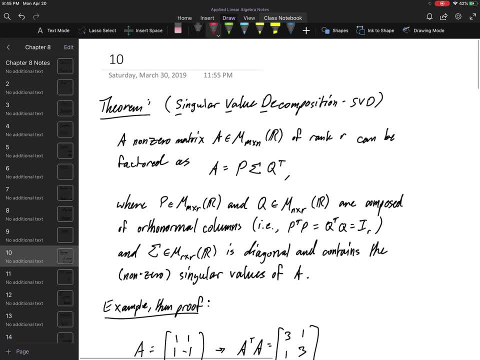 that there probably is a slick way to do this. So let me show you. We have the following theorem that shows us how to break up these pieces, or tells us what these pieces look like. So this is our singular value: decomposition theorem. 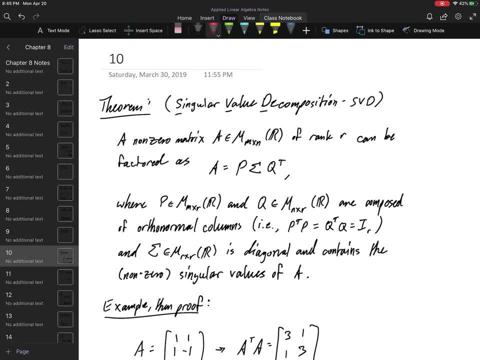 So a non-zero rectangular matrix, A with rank R, can be factored into something that looks like P times sigma times Q transpose. So we're very close. A looks kind of like sigma times Q transpose, but there's this extra factor of P here. 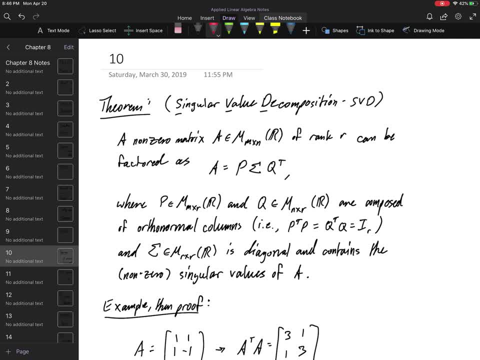 And P is an M by R matrix and Q is an N by R matrix. These guys are composed of orthonormal columns, right? So these are not orthogonal matrices because they're not square. However, they do behave like orthonormal or like orthogonal matrices. 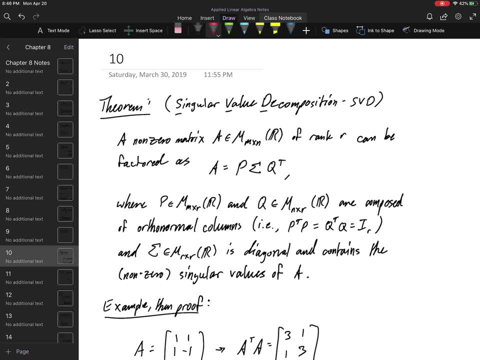 at least in the P transpose P and Q transpose Q departments. So we also have a matrix sigma which is effectively acting as the square root of the diagonal matrix. the diagonalization of A transpose times A, And this sigma is going to contain the non-zero singular values of A. 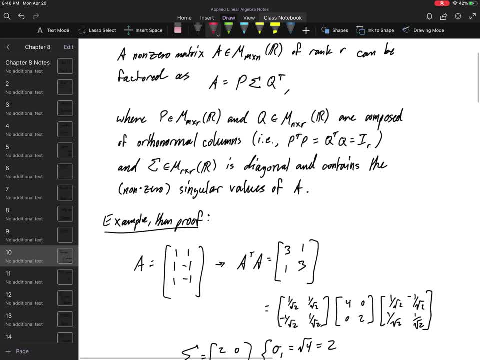 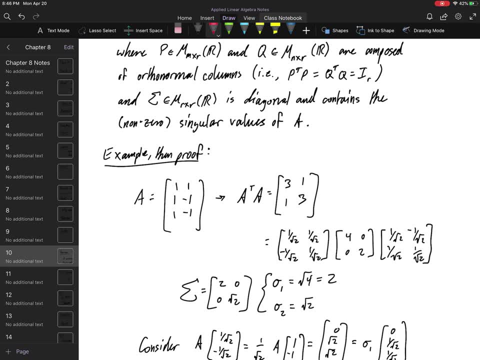 So, to give you an idea of why this might be the case, let's walk through an example. right- And this was the A that I gave you just a moment ago- in MATLAB, We can go ahead and compute that A transpose A. 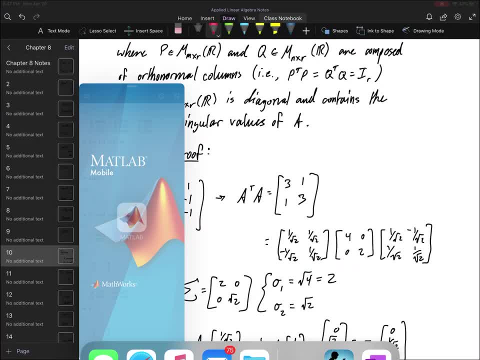 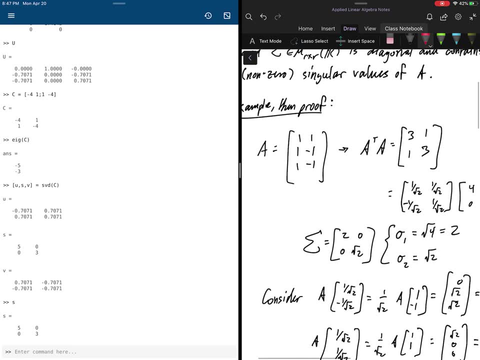 You know what? I can go ahead and verify this. Let's go ahead and just keep this guy. Oh, there we go, Come on. Okay, Let's go ahead and keep these examples on the page. So, coming back here, 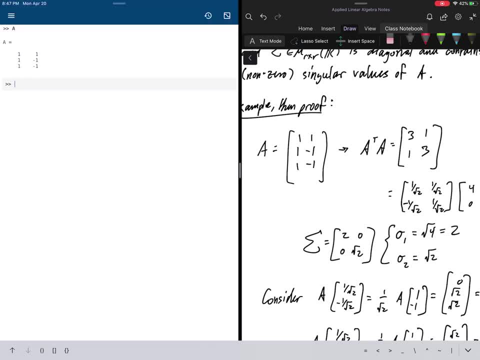 let's clear the screen. A, just to remind you. yes, that is the correct thing that I have in MATLAB And we can compute A transpose. A is indeed. ooh, I wrote it down wrong in the lecture notes. Shame on me. 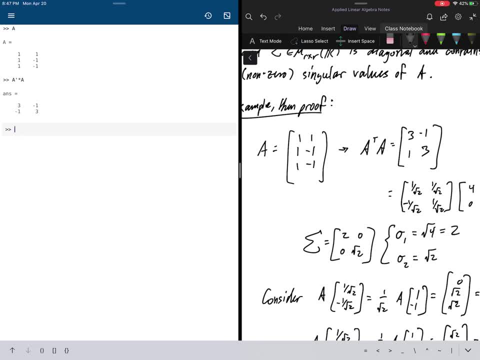 Yep. So let's go ahead and fix that. Do do, There we go. So it's three by minus one by minus, one by three. However, I can go ahead and create what MATLAB calls the singular value decomposition And 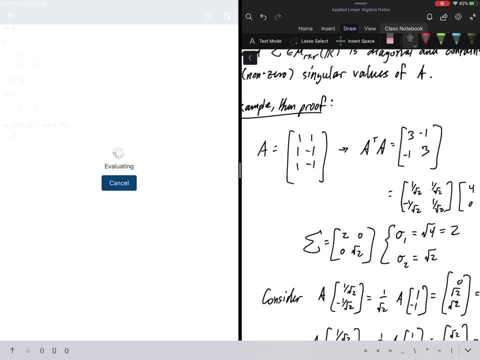 it will be A transpose. A will be given by these matrices. Now you might see numbers that are very similar, that are like up to a negative sign, just to make sure that they are symmetric, because MATLAB likes symmetric things. 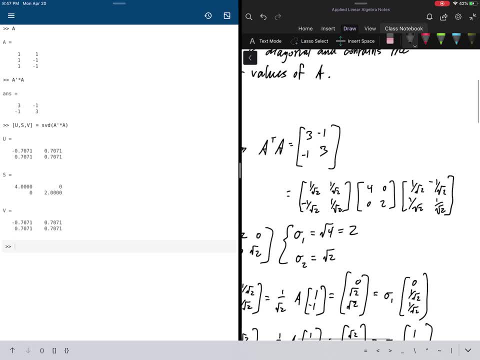 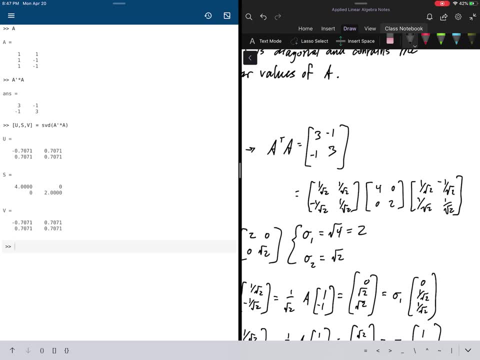 just as well as it likes rectangular things or square things, But the point is that I can go ahead and break this guy up into the following decomposition: Right? So this is exactly the fact that A transpose A is. 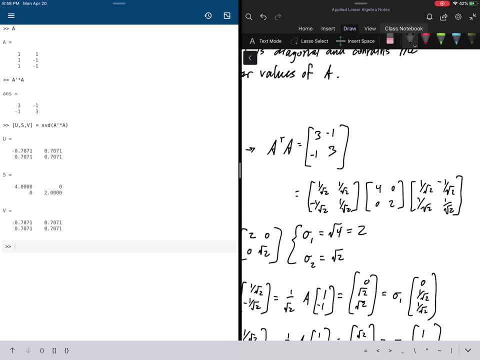 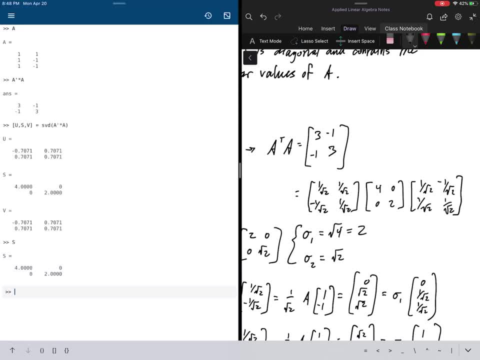 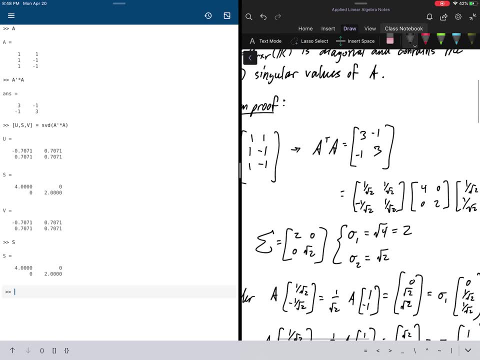 Yep, But the point is S here is composed of- well, it's supposed to be this square sigma matrix. So if I take the square root of this guy, I come up with sigma, And sigma is going to be two by root two. 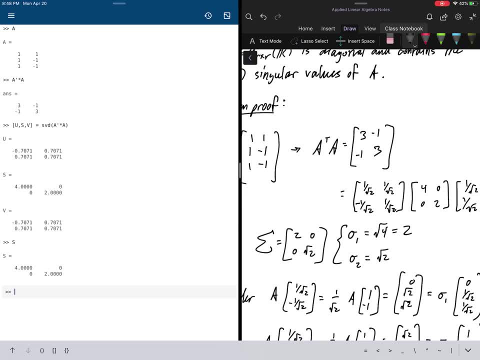 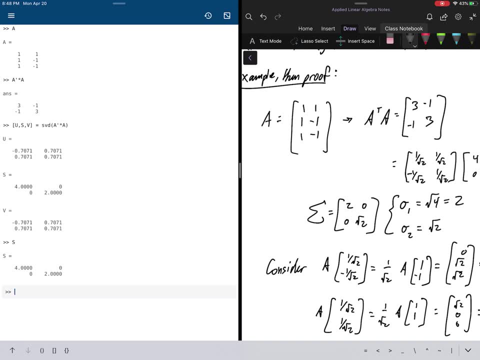 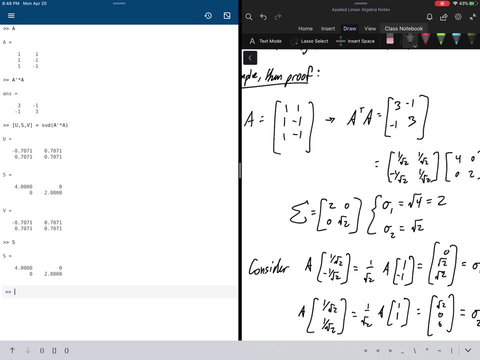 down the diagonal of a two by two matrix. Okay, Okay. so notice, this is a two-dimensional or two-by-two matrix, but A itself is a three-by-two matrix. so that means that sigma is really going to be a square matrix that's given by or whose. 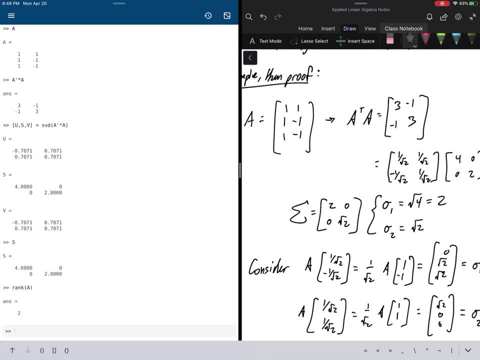 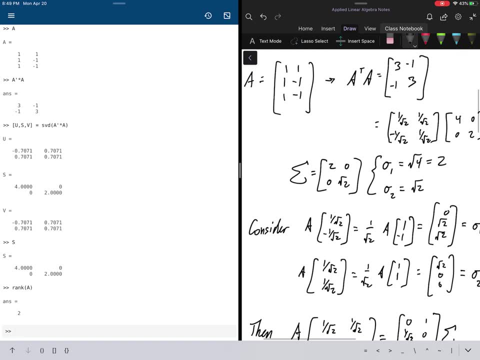 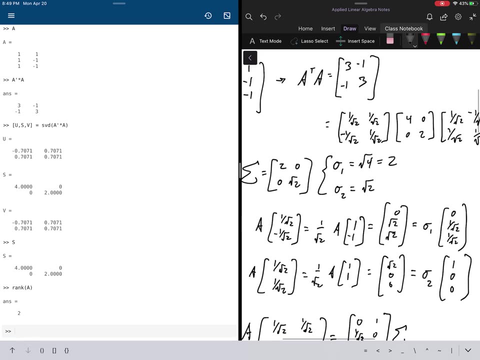 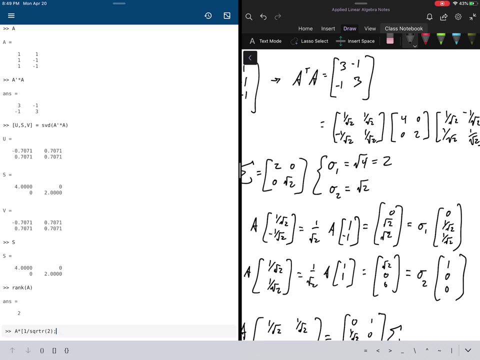 dimension is given by the rank of A, and I can double check that The rank of A is indeed two, All right, so that's why we have a little index r standing for rank. So notice what happens here If I do take A and multiply into it. so A star one over square root, two by negative, one over 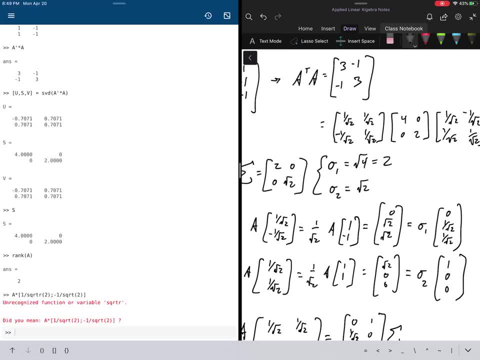 square root two: Oh, come on. Oh yeah, that means I just wrote it down wrong: Squirter, No squirt. Oh yeah, squirt, not squitter, Squatter, Squirt. There, it is Notice that we wind up with. 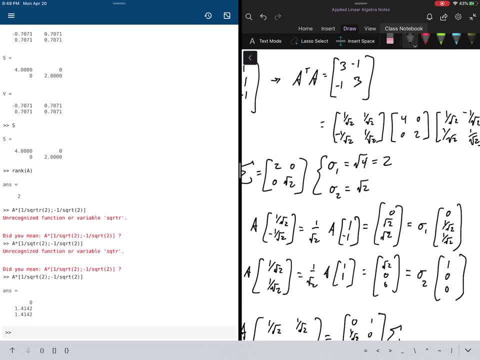 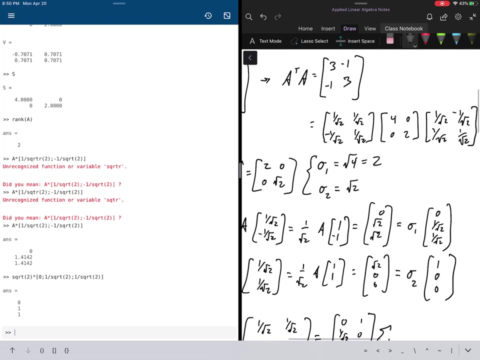 A Something that is a singular value times a unit vector. So this is square root of two times the vector zero by one over square root. Oh, come on, One over square root, two by one over square root, two, And sure enough, that's exactly this. It's going to be some. 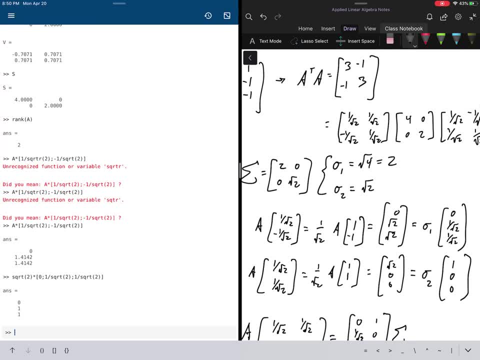 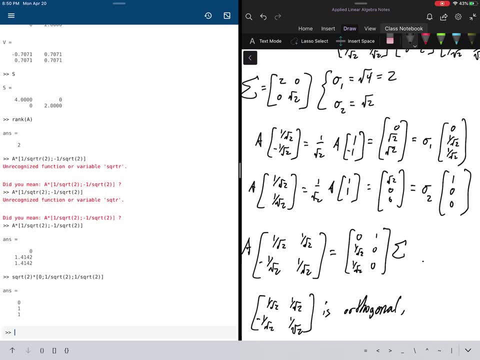 matrix that I want to use here. It's going to be effectively one of my principle vectors. So this new vector here, zero by one, by one, is acting like an eigenvector for A, since I can go ahead and factor out a singular value from this guy and get a unit vector. 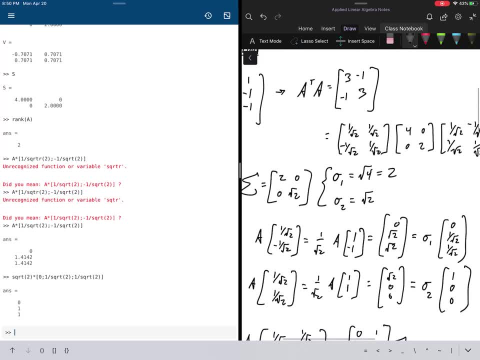 in return. Notice that I get the same thing. By the way, I'm getting these guys from up here. Okay, so this guy goes down here, This guy goes down here. So these, I'm not just pulling these out of thin air, I'm just making sure that when I multiply A. 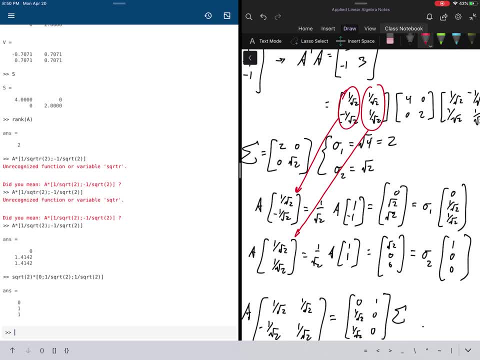 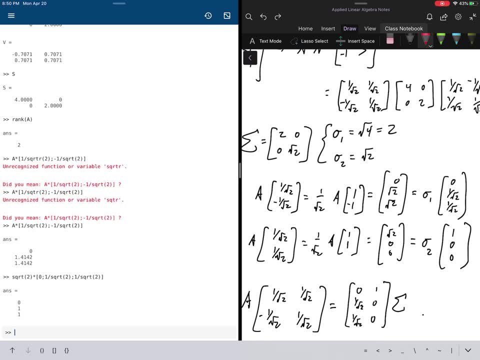 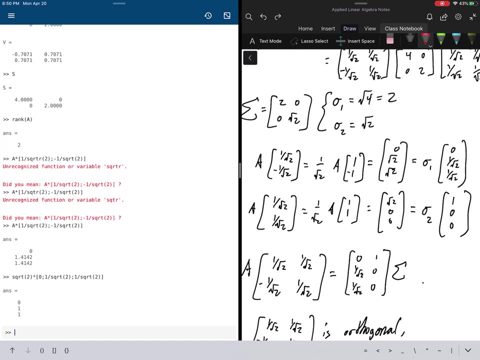 into these vectors that I wind up with something that makes sense, something that looks like an eigenvector. And sure enough, if I multiply A into one over root two, by one over root two, then I can go ahead and factor out another singular value here and come up with a unit. 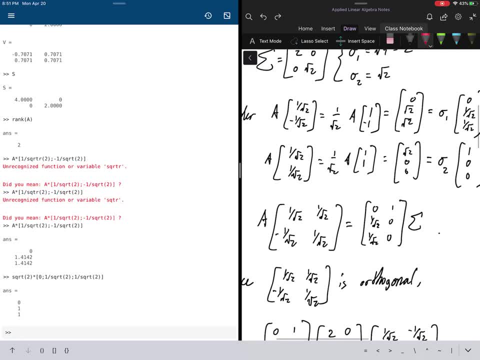 vector one zero, zero on the outside. So that means if I throw those two opposite sides I'm going to get a unit vector one zero, zero on the outside. So if I put those two operations together into one matrix multiplication, 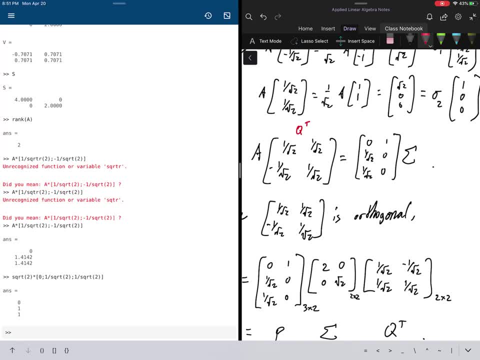 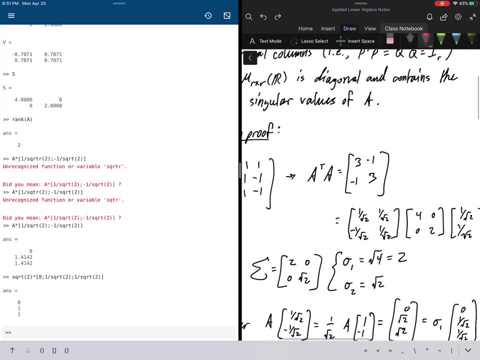 I wind up with A times, this is effectively Q transpose. and then I wind up with: is it? No, This is the Q that I want. right, Because I want, yeah, I want a Q transpose at the end of this. 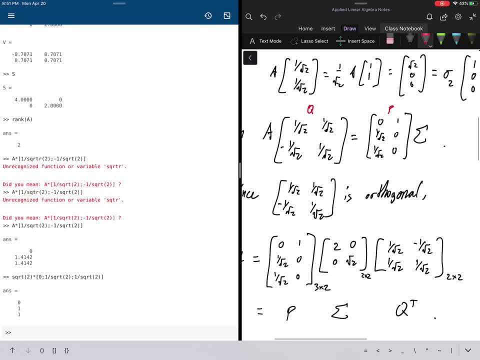 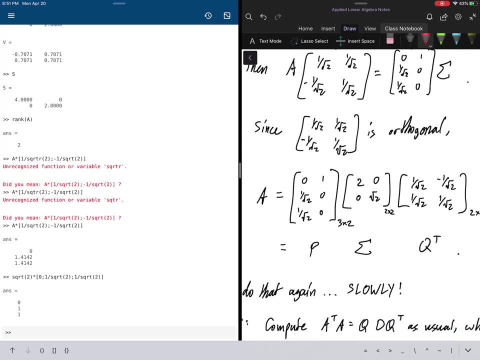 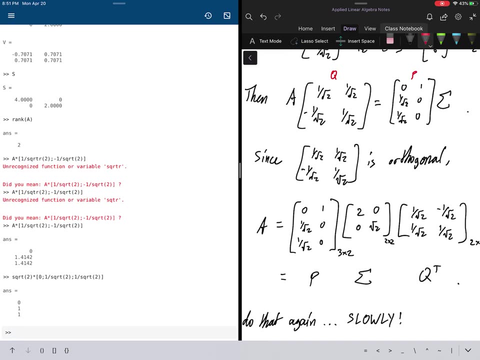 And this guy I'm going to go ahead and call a P, right, This is going to be my principal vectors: P for principles. So notice what happens here. Because this matrix Q is composed of an orthonormal basis of columns, it's an orthogonal matrix. 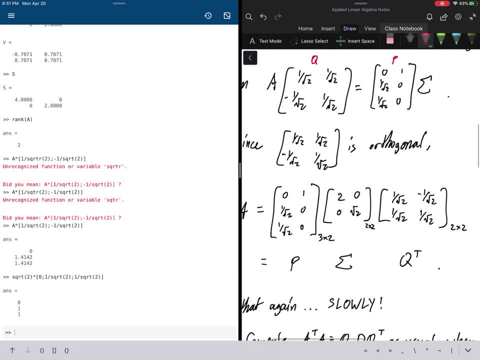 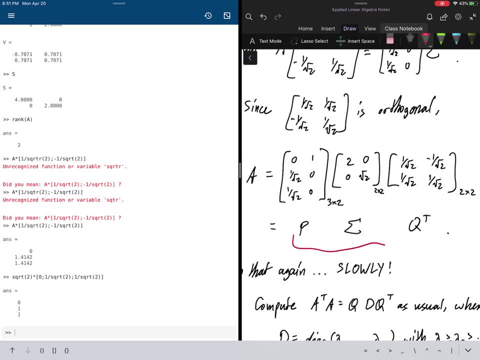 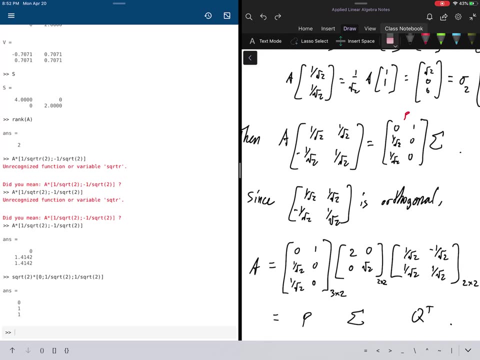 so that means that its transpose is equal to its inverse. So I can go ahead and flop the Q over to the other side at the cost of adding a transpose, And this is exactly the decomposition I was looking for. Okay, so there's the proof of concept: This does work. 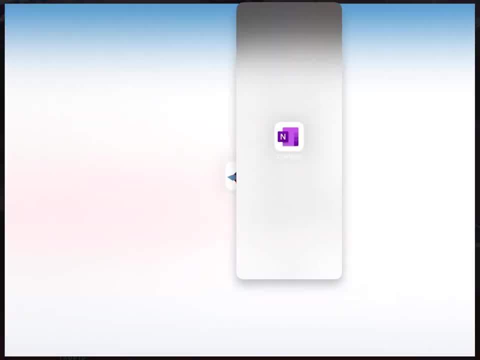 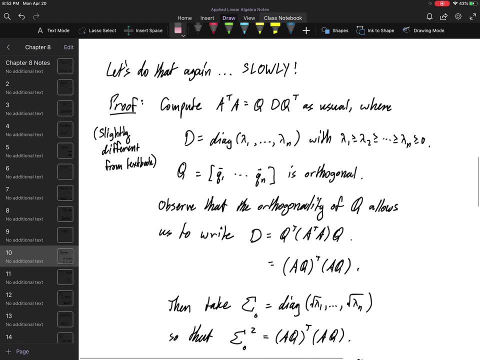 We can do this. Let me show you how to do it more generally, to show you that it it actually does still work in the general setting. So let's do it again, very slowly. First step here is to go ahead and compute a diagonalization of A, transpose A into. 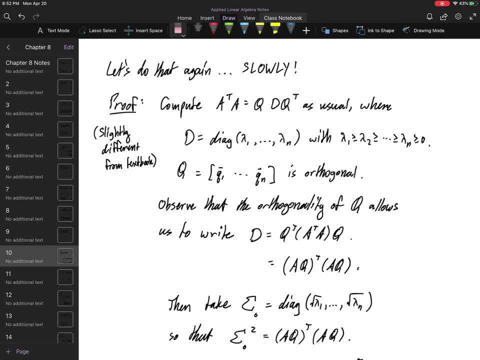 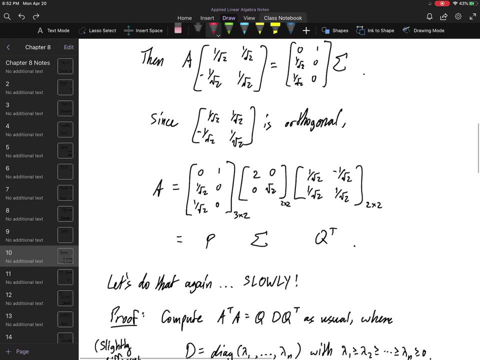 orthonormal eigenvectors. So this will give me a full n by n decomposition, or set of n by n, matrices, Q and Q and D along with Q transpose. So notice at the end here there very well could be some eigenvalues that are equal to zero. It is okay, That's not bad just yet. 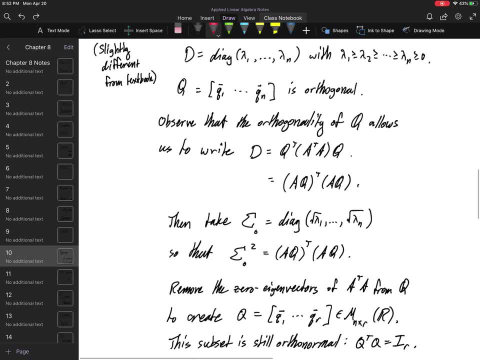 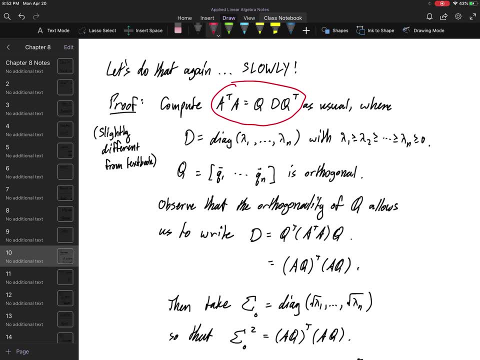 So what we're going to do is observe that, through orthogonality, this relationship here will allow me to rewrap these, to rewrite D in the following way: I can go ahead and take the Q here, multiply on the left by a Q, transpose and then take this guy, multiply on the right by a Q and I'll wind up with an. 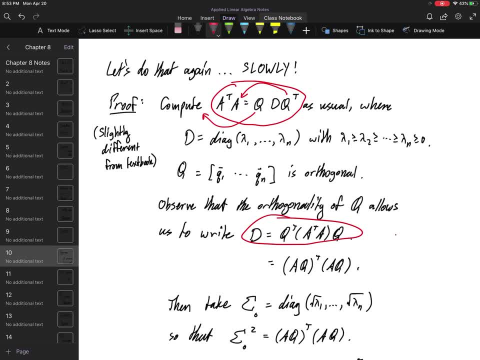 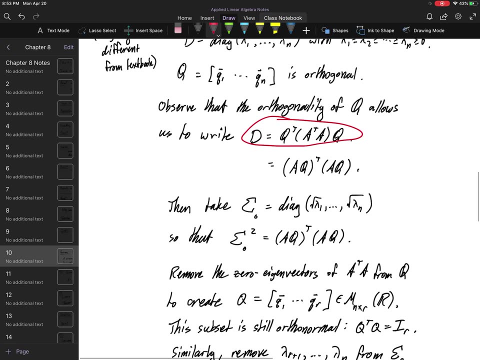 expression for D? Right, we've seen this before. This was effectively our S inverse A S decomposition for a diagonalizable matrix. So no problem there. This is the same exact thing, right? It's nothing new yet. And what we notice at this point is that I can go ahead and break this guy down, not into. 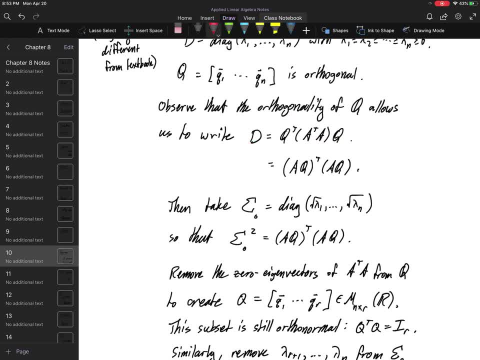 the associated matrix, the association I have right now. I can reassociate these parentheses and notice that A Q transpose shows up on the left and A Q shows up on the right. So awesome, That's looking more and more like something that we want. 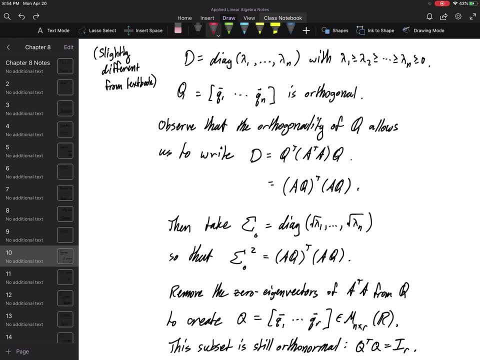 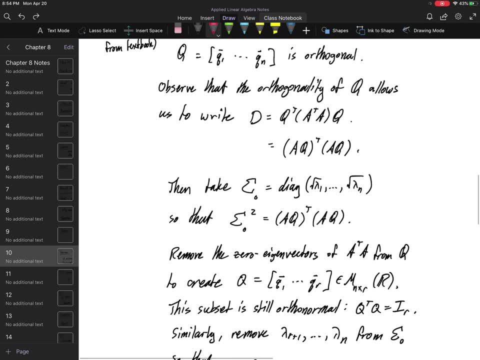 But then we take a look right, We have a whole bunch of extra potential, zero eigenvalues that we need to get rid of. So this sigma I'm going to take to effectively be the square root of D. right, This is what we were doing before, So that D is actually equal to this guy. 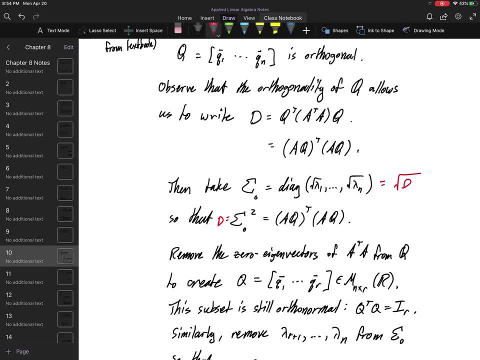 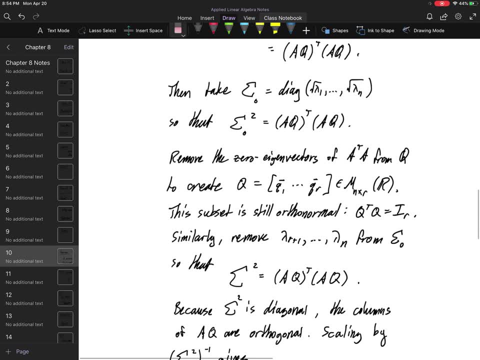 D equals sigma zero, squared right. That's exactly what I want: Two, three, four and get rid of that one as well. And from this sigma, from this sigma zero, we're going to remove all of the zero eigenvectors and 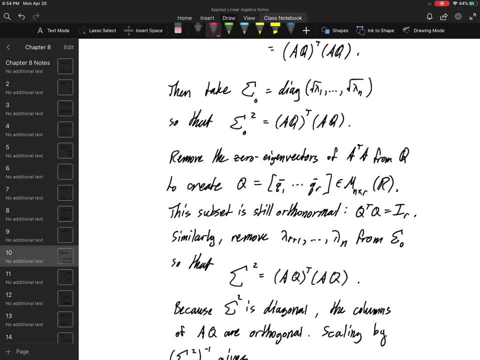 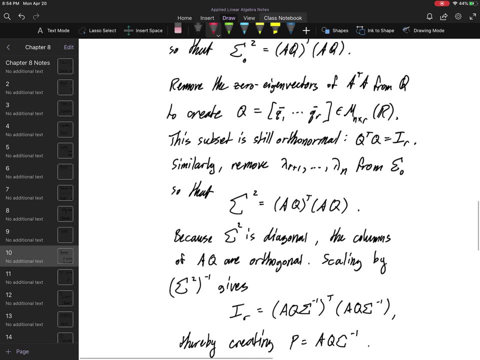 eigenvalues. So from sigma zero we're removing eigenvalues and from boldface Q we're removing the basis on the null space. So this subset, because it came from an orthonormal set, is still orthonormal. Therefore, Q transpose Q, this new Q, right, This guy where I took away all. 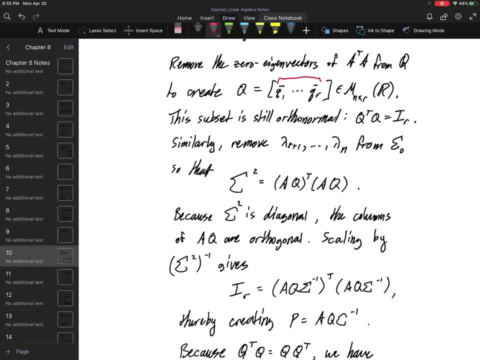 the zeros, like all the nulls, and I took away all the zeroes, I took away all the a's, I took away vectors. Take those guys, put them into one matrix. call it a regular Q instead of a boldface Q. 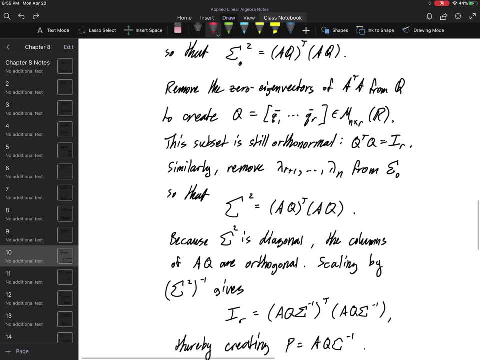 and we're going to wind up with something that behaves like an orthogonal matrix, even though it's not a square matrix. So, very similarly, we're going to remove the lambdas R plus 1 through Rn, or lambda R plus 1 to lambda n from sigma 0,. 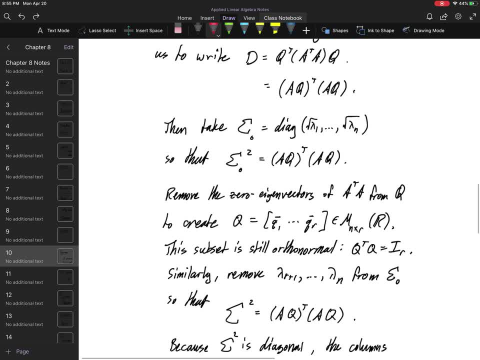 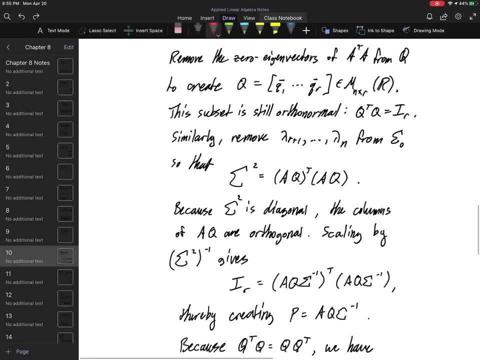 because I know that there are that many, because R is the rank of this matrix and anything beyond that is going to be contributing to the kernel. So that means I have an n minus R dimensional kernel. so I need to get rid of that many singular values, which means I need to remove those eigenvalues. 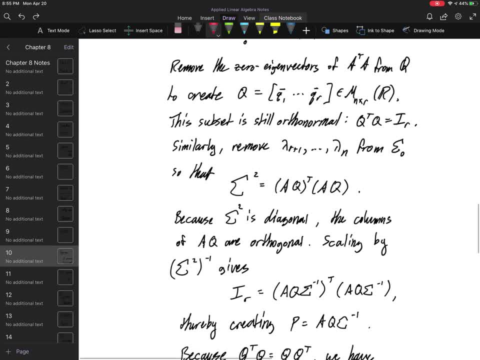 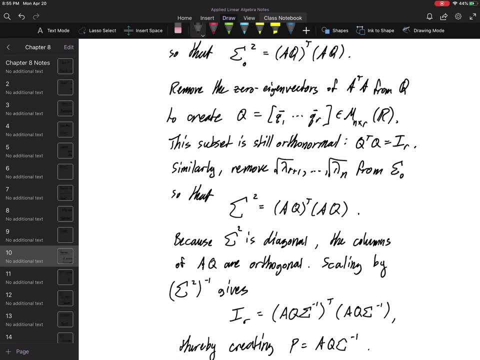 from sigma 0.. And technically these would be square roots. is that right? Yeah, these are square roots. Let me go ahead and fix that Square root square root, But technically, yeah, screw it, they're all 0 anyway. All those are. 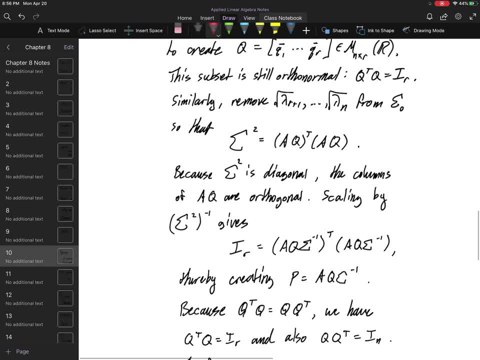 all those are 0 eigenvalues, So that sigma squared- here- if I took away all the 0 eigenvalues then I wind up with sigma squared- is equal to A times Q. transpose times A times Q right. Notice, this is actually smaller right. There are fewer vectors in this Q matrix as opposed to. 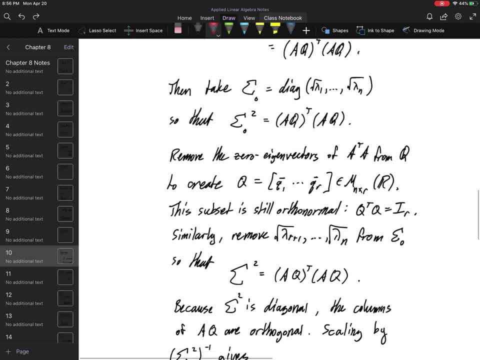 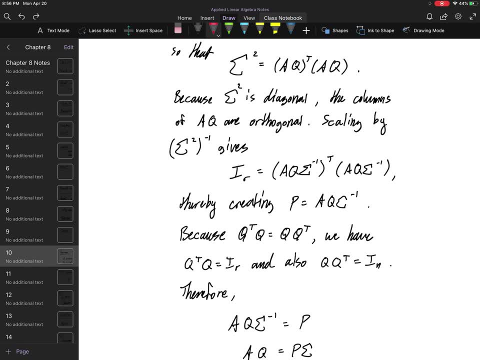 the one that I had upstairs. okay, I am less n minus R vectors from my null space. So because this sigma squared is diagonal, the columns of A times Q have to be orthogonal. right, It's not orthonormal, but all the off-diagonal entries of sigma squared are telling. 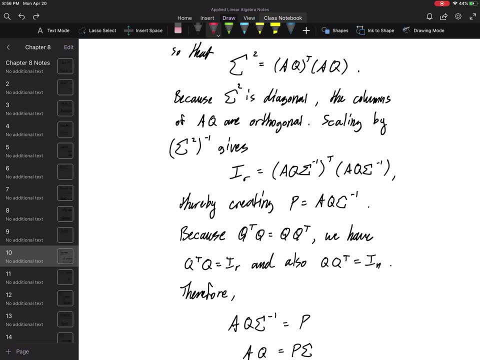 me that the dot products, the Euclidean dot products, between the columns of A times Q must be 0. So the only problem is that the columns of A times Q have to be orthogonal, right? So the only place where they're non-zero is on the diagonal. So this is an orthogonal set of vectors that make 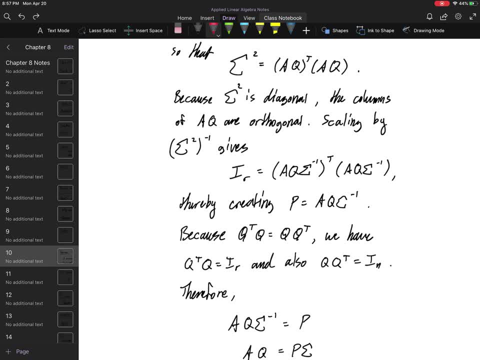 up the columns of A times Q. So once I'm here, I can go ahead and scale this guy down by effectively dividing, effectively dividing a sigma on the left and on the right, so that I wind up with this fellow. And this is effectively what we're going to take to be P right. So P is actually. 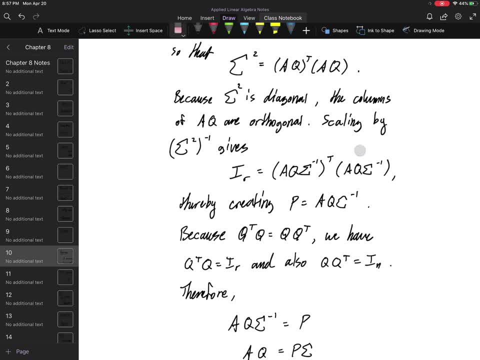 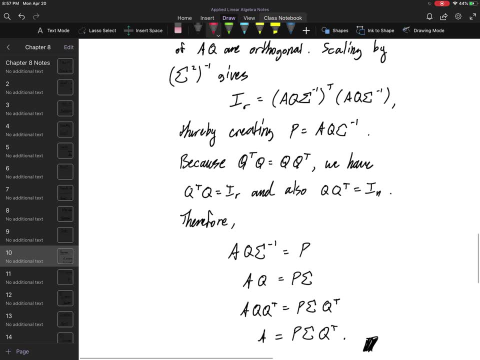 something that we don't get from the diagonalization up front. It's something that we have to create from the diagonalization of A transpose A. So these vectors are actually fairly costly to produce, but there are nice algorithms to get them quickly, So we thereby create the matrix P. 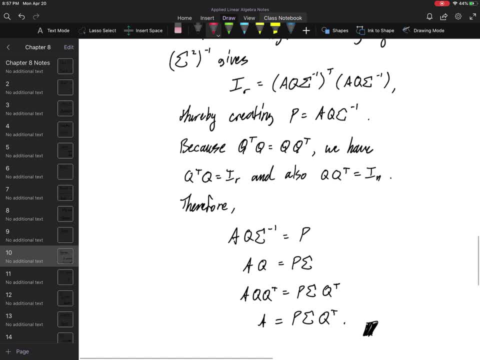 and that's A times Q, times sigma, inverse right. Because I know, because the fact that bold Q was an orthogonal matrix. not only do we have that Q transpose Q and Q Q transpose are equal to the identity matrix, they share this property with Q transpose Q. So the little, the regular. 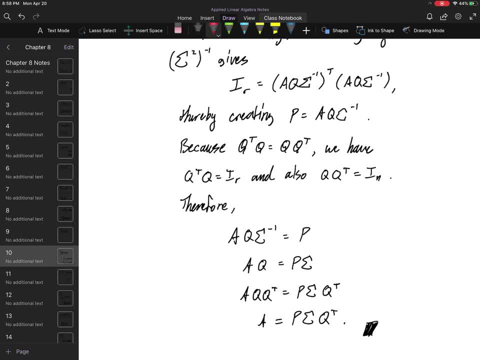 typeset Q as opposed to the boldface Q, Not only do I get the Grom matrix between an orthonormal set of vectors, but if I go ahead and reverse that, the projector matrix is actually a larger matrix, but it has it's- the identity matrix. 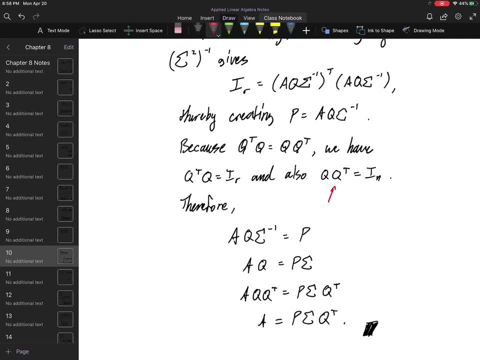 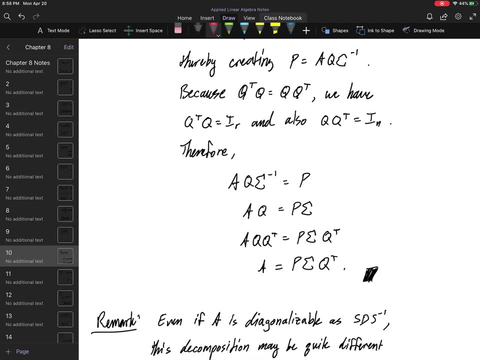 This is the identity matrix and I think it's actually, up to a certain point, like there would only be R, non-zero entries in this guy. But when I think about that, is that right? No, it actually fills it up. It actually does give me the identity matrix. So at the end of the day, 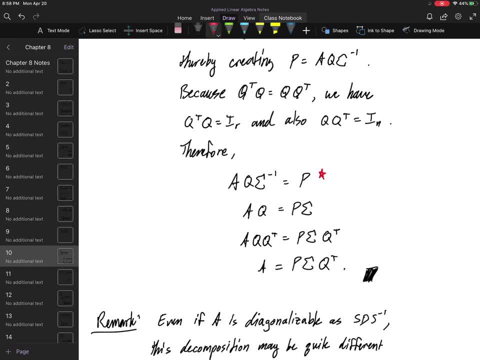 what we wind up with is the fact that P is defined thusly: I can go ahead and multiply the sigma on the right, I can multiply the Q on the right by or by a Q transpose. That way these guys go away into an identity matrix and I wind. 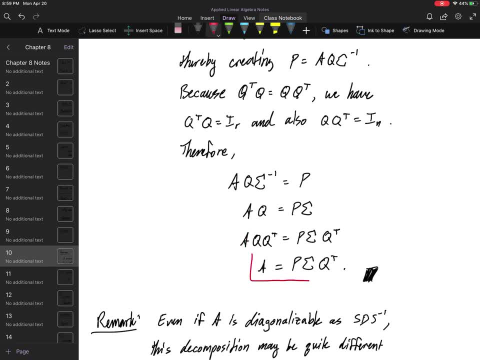 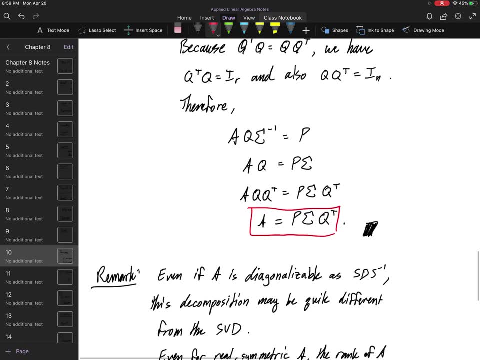 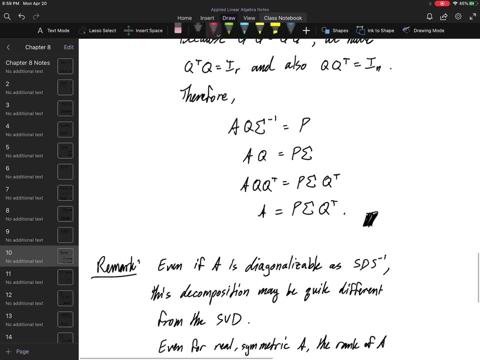 up with what is known in the trade as the singular value decomposition of A. All right, So there is a way to break this guy up. even if it's not square, even if it's not diagonalizable, there is a way to break this guy up. 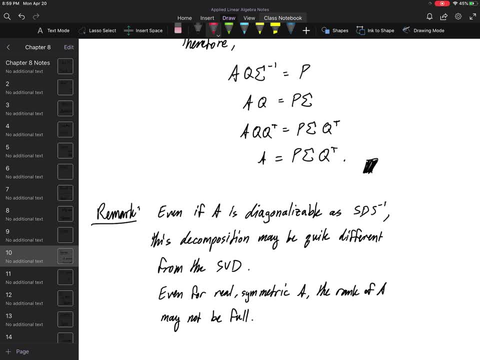 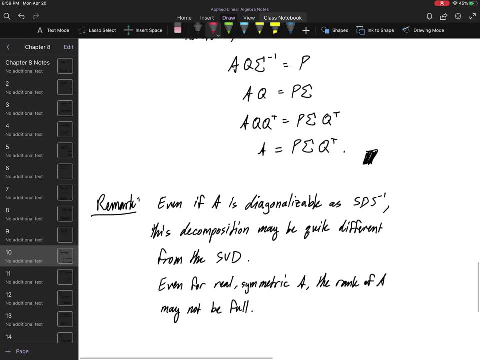 So that he looks diagonalizable, that we still wind up with the same sort of geometric properties that we did in the previous video. And, more to the point here, if A happens to be diagonalizable, then, yeah, we do wind up with something that looks like a diagonalization, But we made the 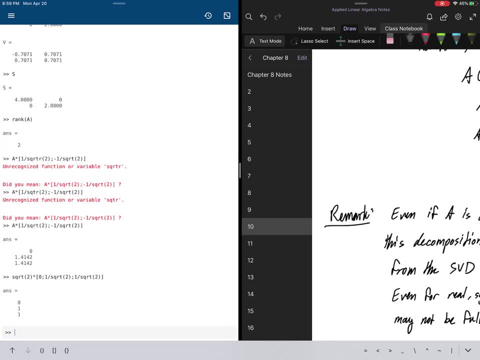 comment earlier that the SVD is not the same thing as a diagonalization. We had that matrix C to show it to us. So if I checked the eigenvalues once more for C, they're negative and I'm going to write that as negative. But if I wind up asking for the SVD of C, it's just going to give me the. 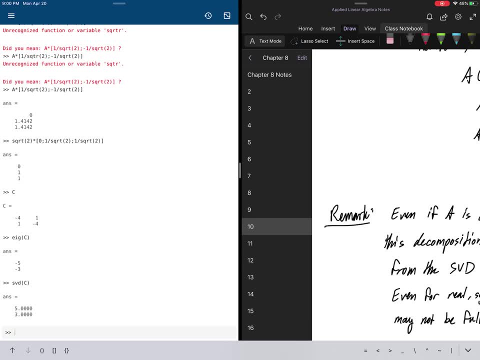 singular values of this matrix C And those are the absolute values of the eigenvalues of C. So it's not quite the same thing as a diagonalization. It's very close, very closely related. But again it's giving us a way to assign dominance to the diagonalization. So I'm going to write this down in a 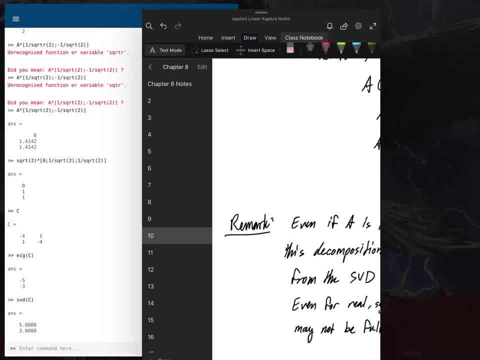 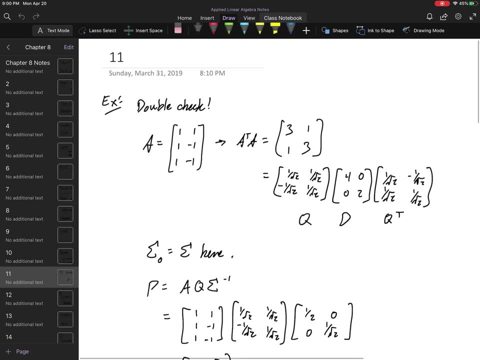 the eigenvalues right. So let's go ahead and finish up this section. I know the video is running a bit long, but bear with me. we're almost out of the woods here And I just wanted to double check that, indeed, the thing that we computed before. you can go ahead and throw this into. 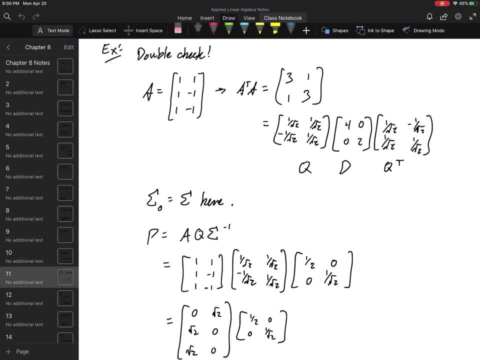 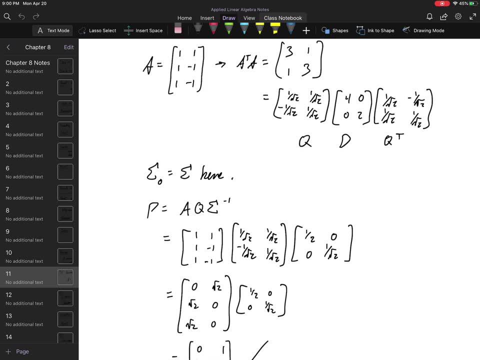 MATLAB. By all means check it out. This guy does diagonalize in the way that we saw before. We can go ahead and create sigma zero by just using the square root of d. right, There's no problem in this case, because there are no zero eigenvalues. right, There are no zero eigenvalues. 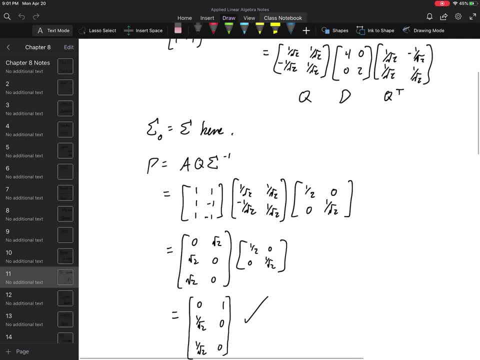 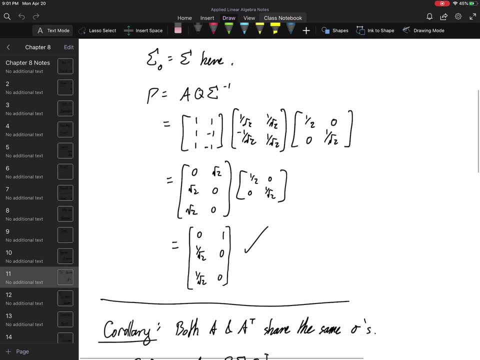 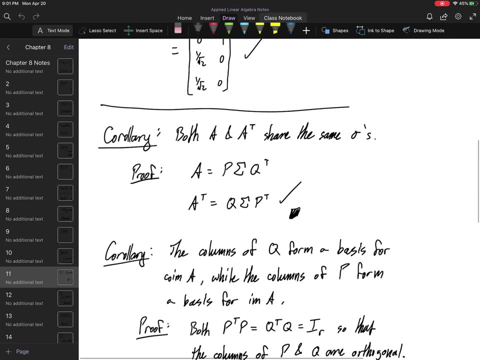 for this guy. So p is just going to be whatever this matrix, a is times, q, times sigma inverse. And there's the p matrix from before. We do see exactly the same thing, right? And the last thing to talk about before we stop that section, before we go into: 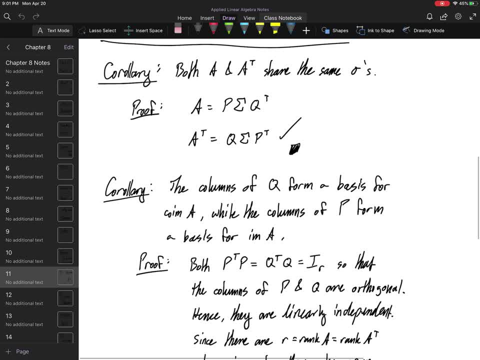 application. Some things to note. a and a- transpose- share the same singular values, but they don't necessarily share the same principal vectors. In fact they're kind of opposed to each other. They are transposed versions effectively. So the singular vectors I get in a are actually the columns of p. 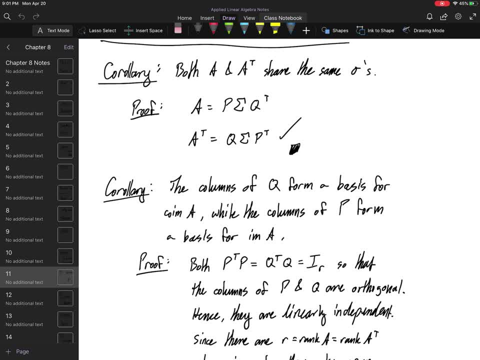 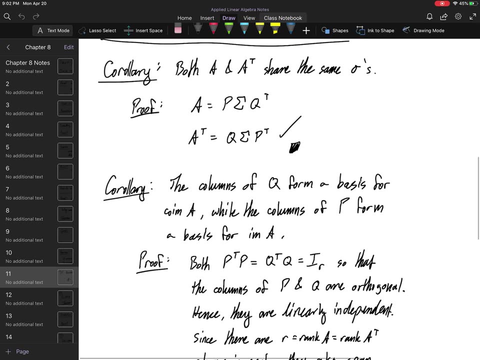 but the singular vectors that I get for a transpose are actually the orthogonal matrix q or are the columns of the orthogonal matrix q Or the thing that looks like an orthogonal matrix? Both p and q kind of look like orthogonal matrices, come to think of it. But the point is that these guys share the same singular values. 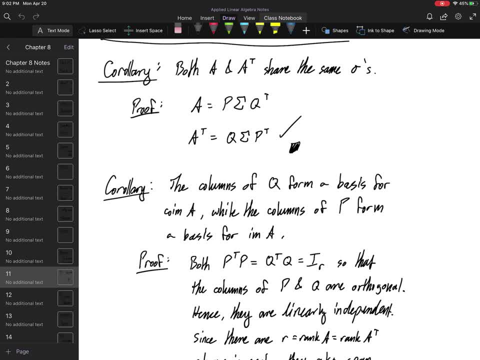 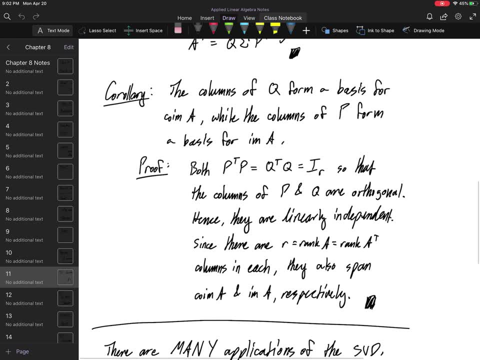 Not necessarily the same principal vectors or singular vectors, but the same singular values for sure. So second corollary is that the columns of q form a basis for the co-image of a, but the columns of p form a basis for the image of a. 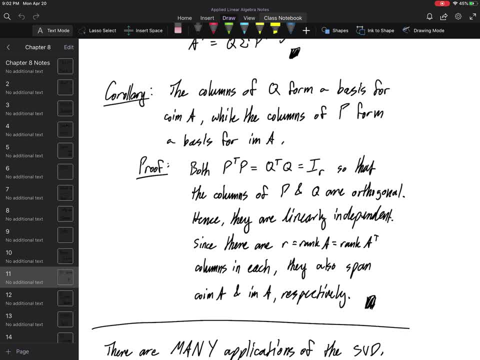 Kind of interesting that that holds up. So that means that q is going to be really helpful for us in figuring out least squares problems, Because I know that my minimum length solutions, or close solutions, no, my minimum length solutions to a system that has infinitely many solutions.